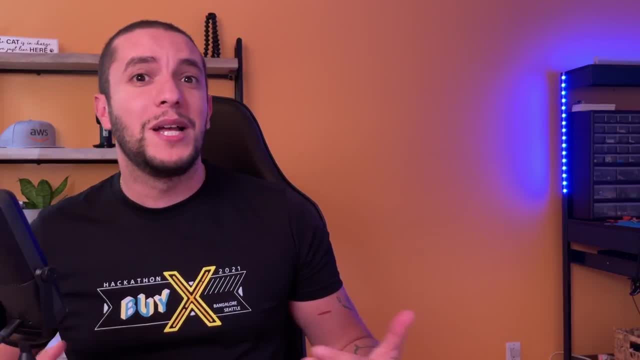 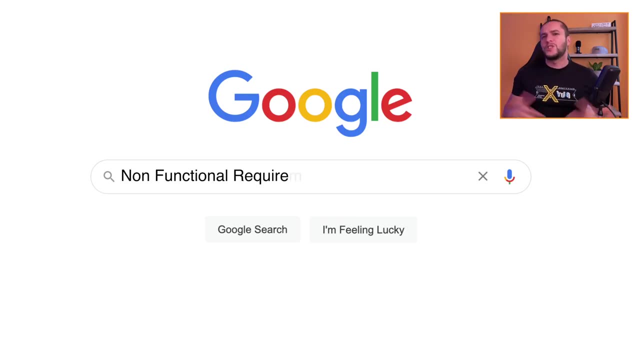 requirements that define what the system is supposed to do, But also- and that's the part nearly everyone misses- you need to understand the non-functional requirements. So what are non-functional requirements? And here's what Wikipedia says: A non-functional requirement- 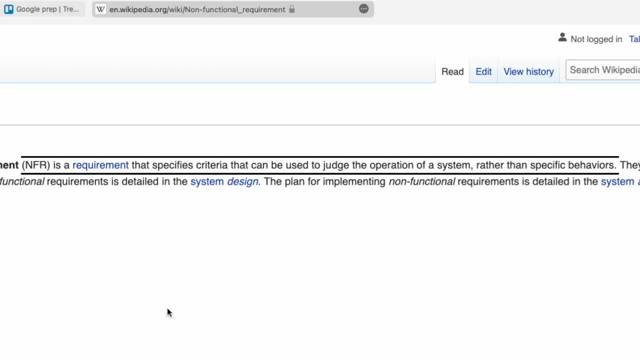 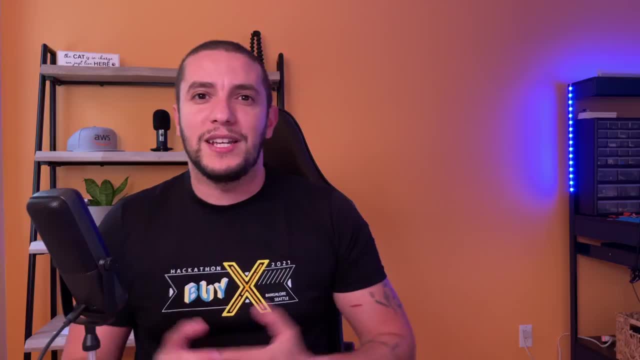 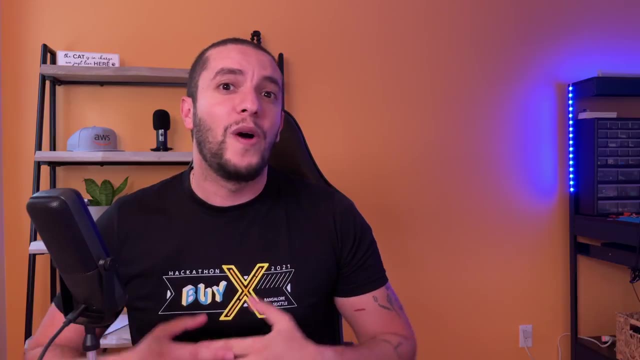 NFR is a requirement that specifies criteria that can be used to judge the operation of a system, rather than specific behaviours. In other words, NFRs define how a system is supposed to be, in contrast to functional requirements that define what the system is supposed to do. 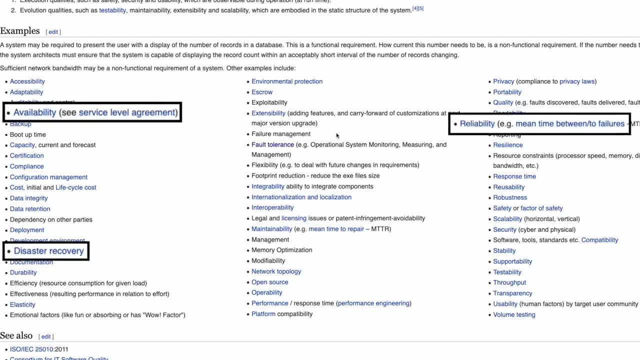 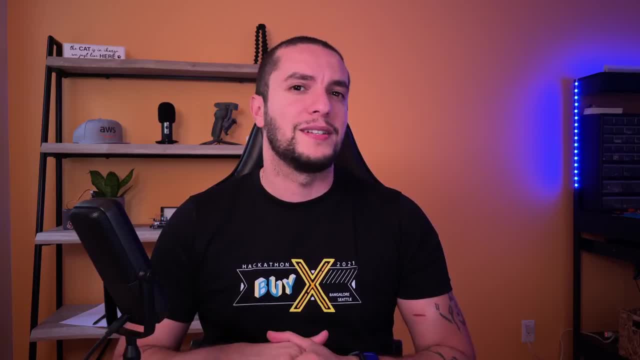 And always on the Wikipedia page. we get already a bunch of examples of what constitutes a non functional requirement, And since oftentimes this is an overlooked step in the design process, I thought I'd take the example of the VOD platform and walk through you. 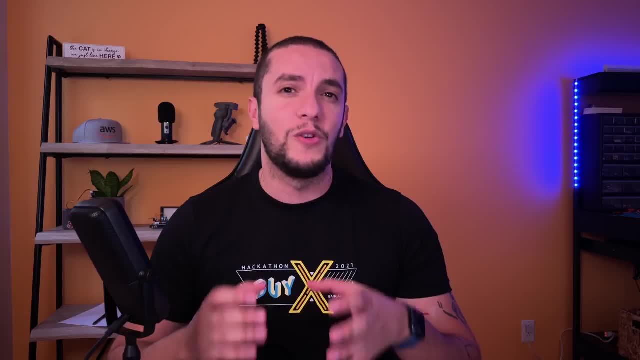 your examples of video on demand for a comprehensive list of what you're supposed to do. to build a comprehensive list of what you're supposed to do- and I will cover the way you can do so- a comprehensive list of requirements we can then utilize to design the first. 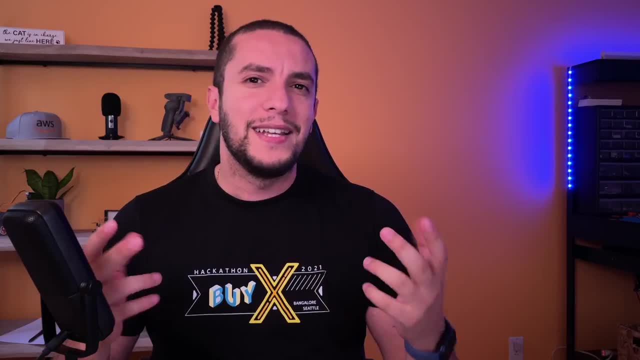 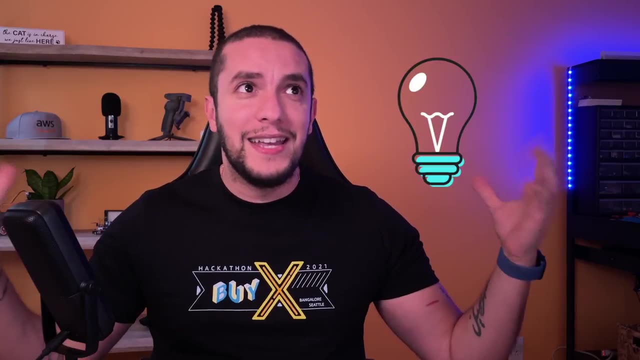 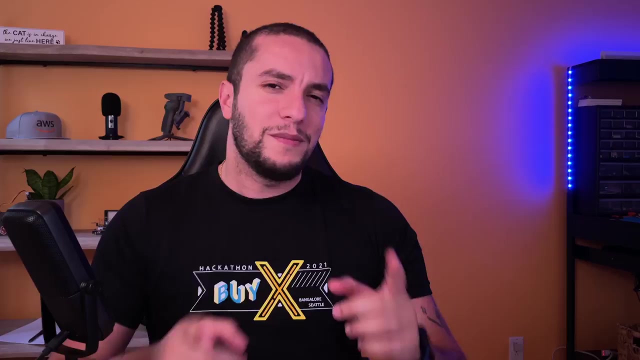 iteration of our architecture. Although I say list of requirements, I saw a previous colleague of mine one day built these as a mind map and a light bulb went on, and I've been using mind maps for my NFR since, and you know what. you'll quickly see why. So let's open up xmind, and this is the software that I 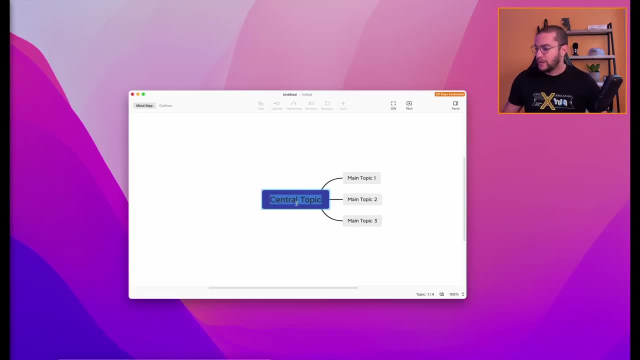 use to build a mind map of non-functional requirements. So I'm just writing the name of the platform- video on demand platform- and here I'm going to be adding a few of the examples that we've seen a bit earlier in the Wikipedia page. We'll start with the reliability and the usability one, and 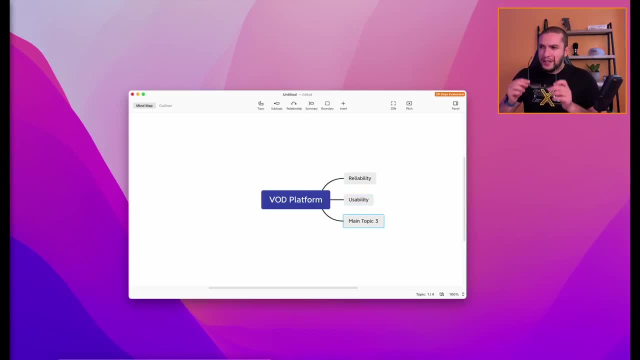 we'll explore a few of them in details throughout the video. I'm going to be adding also a performance efficiency one and cost. of course, I always try to add cost and calculated in terms of money and time. There's portability as well, maintainability, and the last one I'll be adding for this example is gonna. 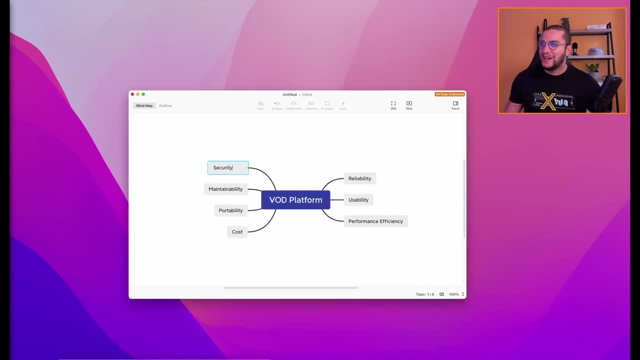 be security and we joke usually because there's a lot of ity at the end. so we joke by saying we're going to be adding a lot of itys. right, There's reliability, usability, portability, security, and the more we dig deeper into these. 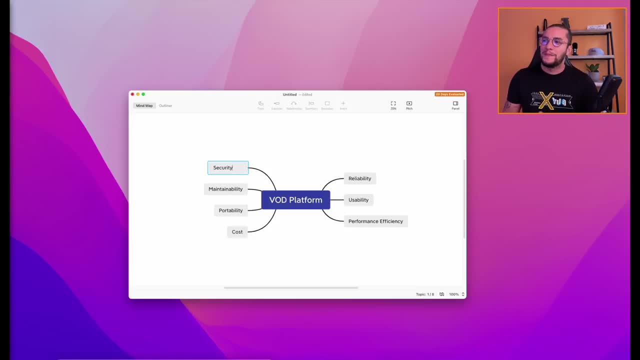 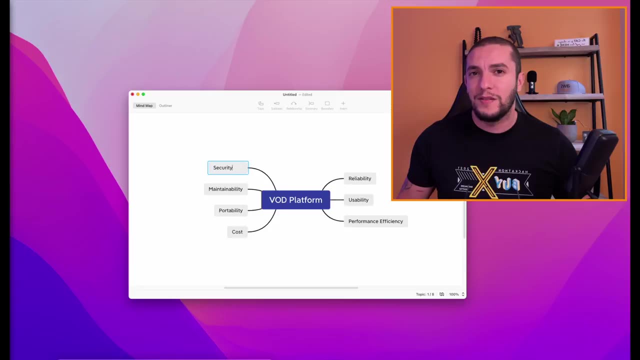 requirements, the more you'll see that more itys gets added as well, And this is, of course, just a demonstration. the goal is just to show you a little bit more about how I go about building a mind map, building non-functional requirements, but, as you can imagine, you can add as many. 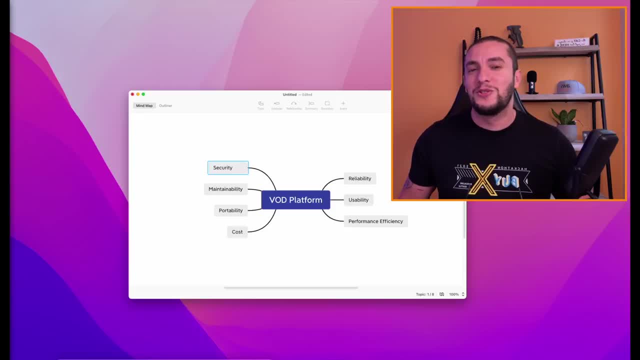 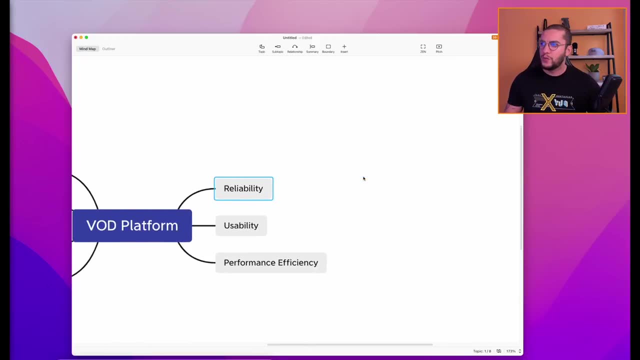 itys as many non-functional requirements as you want to the document to match your own use case. Alright, just zoom in a little bit to make this all clear. We'll start first with reliability. In a nutshell, reliability means the ability of the system to function without a failure, and in order for the system to 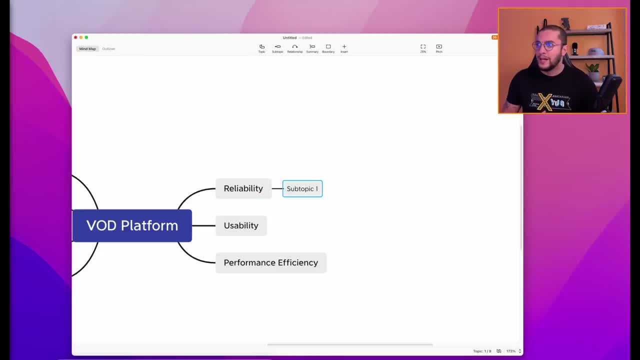 be reliable. there's a few aspects we need to incorporate in our system. First thing is the maturity right: How mature we want the system to be, How available we want the system to be? What about the recoverability aspects of it? What about fault tolerance aspects? And we'll go through these ones one by 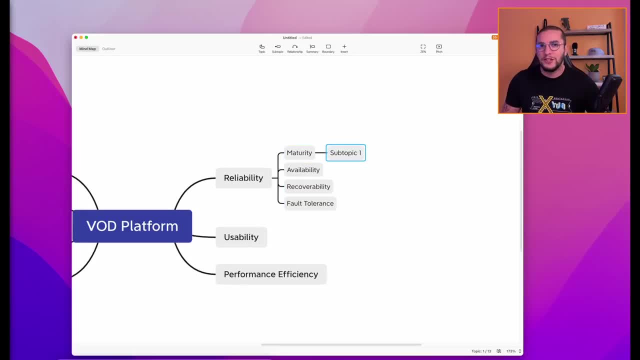 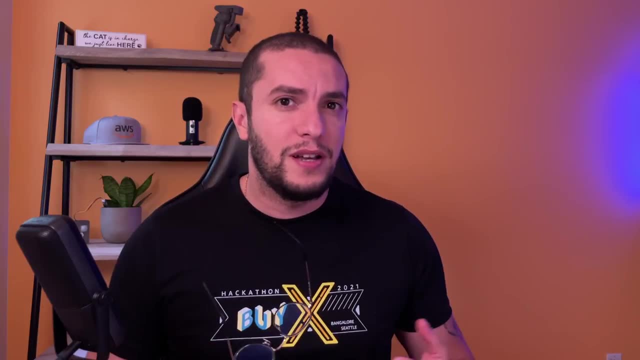 one. So, of course, for video on demand platform, we want it to be functioning 24- 7, and when I say we, it's basically the company or the organization that you are working with or working for, because I don't want you to think that these 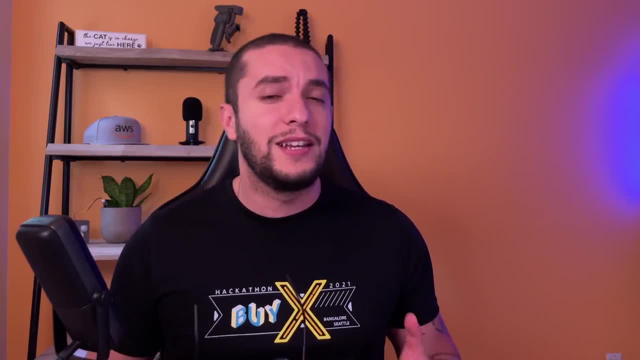 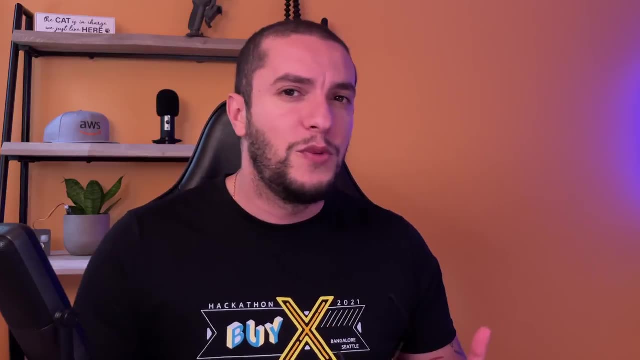 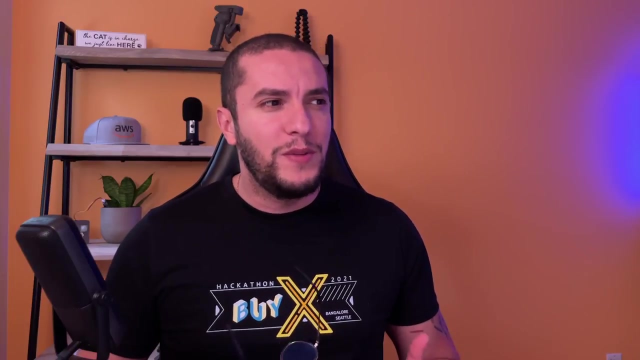 requirements are something that you build or you do sitting in your desk. It's a very pushable requirement and it's gonna take you, realistically, a couple of weeks meeting with various stakeholders- business, people, development, people, ads, people, marketing, people- and with every one of them you're going to be. 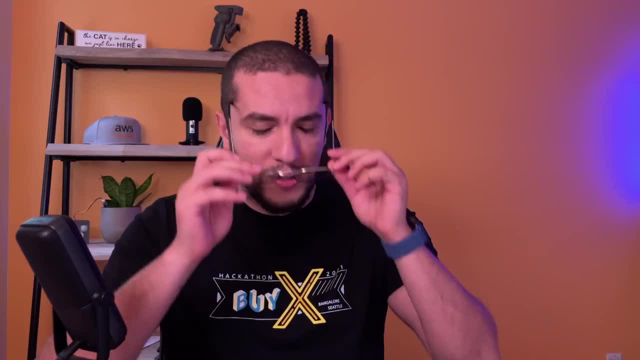 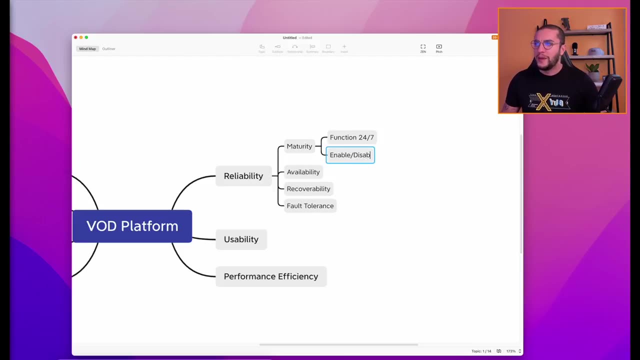 negotiating these requirements. It will become more clear when we'll jump into details. So, of course, we want the platform to be functioning 24- 7.. Something else that I want to add to my platform to make it more mature is the ability to enable and disable features using feature toggling. 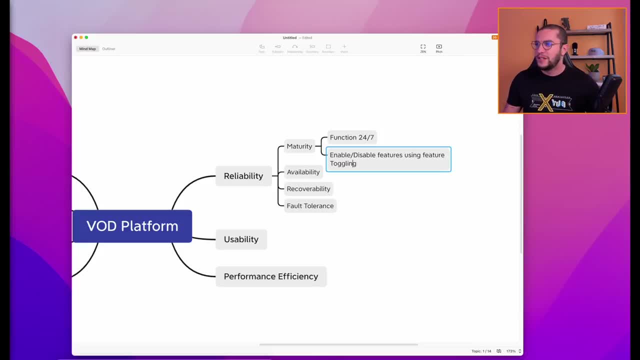 This is usually something that marketing people ask for: The ability to have features ready to go whenever they just click on a button, and we usually do it using a feature toggling. I want my platform to have automated tests right and I also want a side-by-side coexistence of different version of my 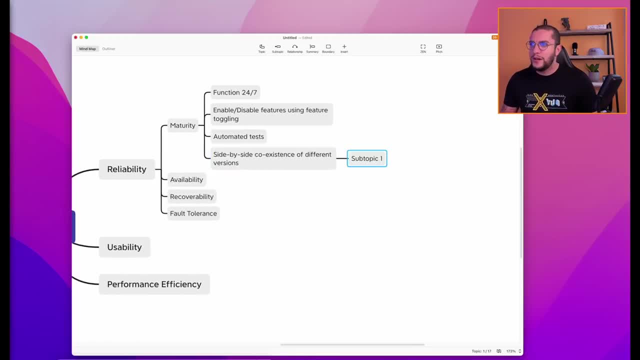 platform. How to achieve that? And you see that now we're going one level deeper. So I want to achieve this side-by-side coexistence by building zero downtime deployments pipelines for all the components. How do I do that? Another level: Maybe by doing blue-green deployments. 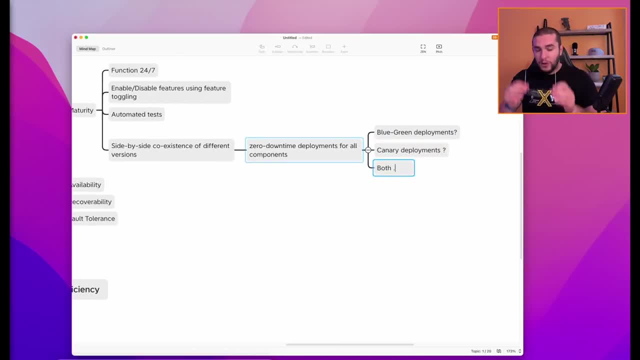 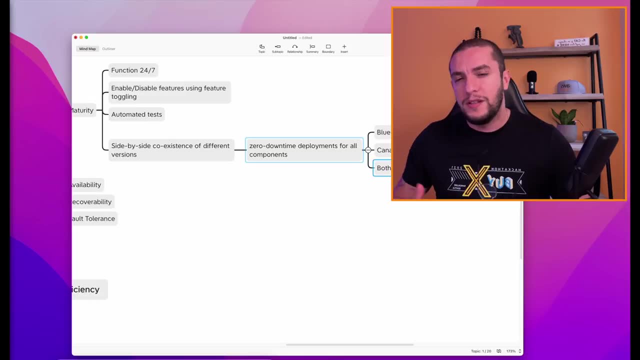 Maybe by doing canary deployments. So this is where you go talk to your ops team, your developments team. If it's developers who are responsible of deploying the application, you go talk to them, you go sit with them and you start negotiating these things. Do you guys need zero downtime deployment? Of course. 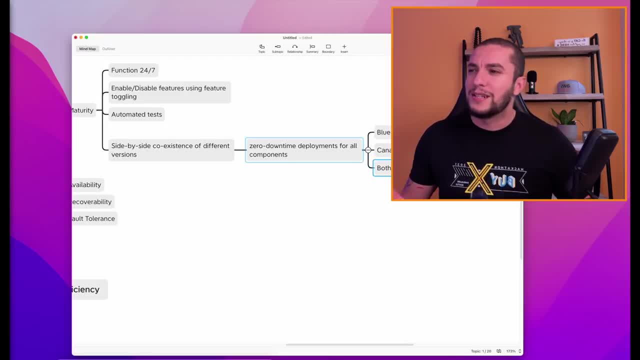 in a perfect world? yes, we do, But sometimes there are other priorities and that's where you start talking to them. Do you guys have experience with blue- green deployments, or maybe you prefer canary deployments with canary deployments? So it's going to depend on the platform, on the company. 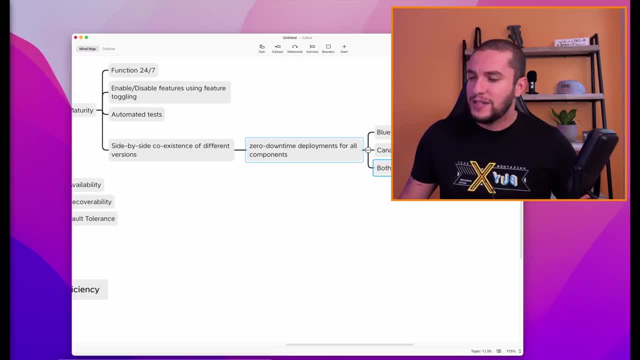 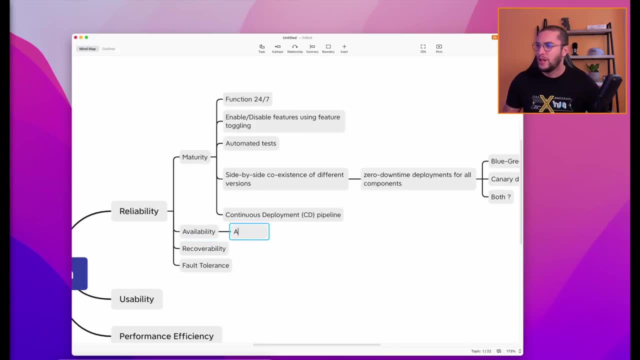 you're working with on the priorities list. So let's keep going. And next let's touch on the availability aspects. Of course, it's a no-brainer: We want the application to be available 24: 7.. Now, what level of availability can we? 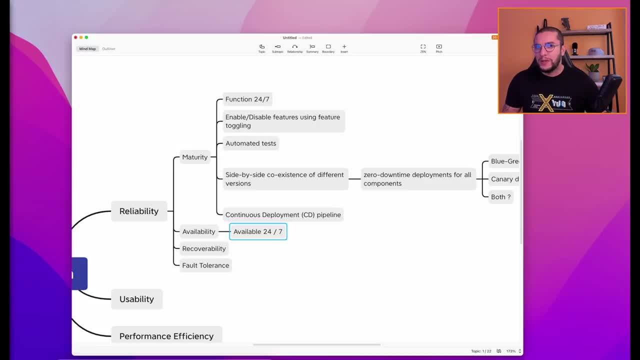 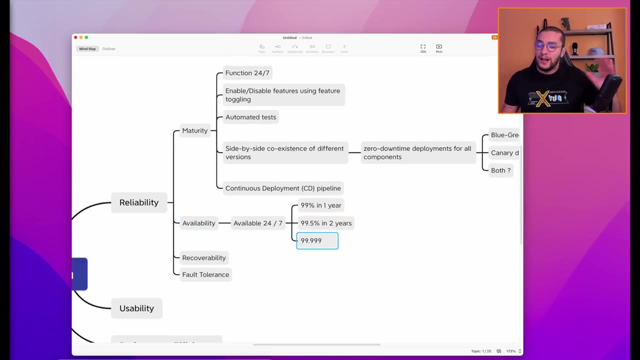 realistically guarantee. As engineers, we believe in iterations, So maybe you will be able to negotiate with your company and 99% availability in the first year And a 99.5% availability in the second year And a 99.999%. 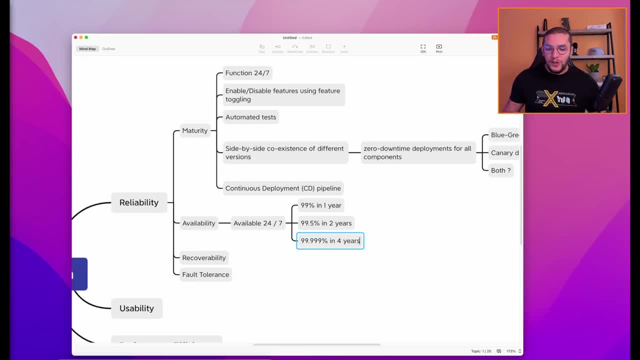 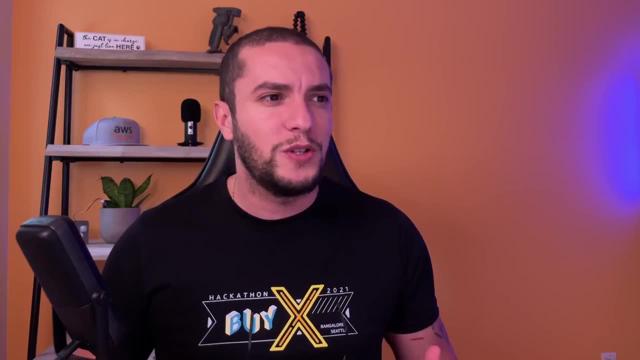 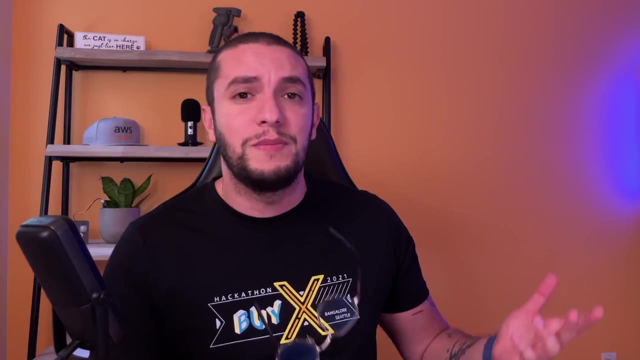 however nines you want afterwards, Because also, again, it depends on the platform- Sometimes spending time and burning through cash and making everyone stressful in order to achieve a level. nines: availability for an internal software that only marketing department use to update pictures of their staff. I don't know, just making examples. So it's not worth it, right? So this is where. 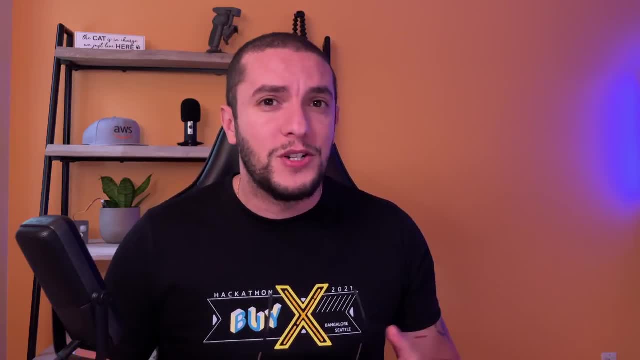 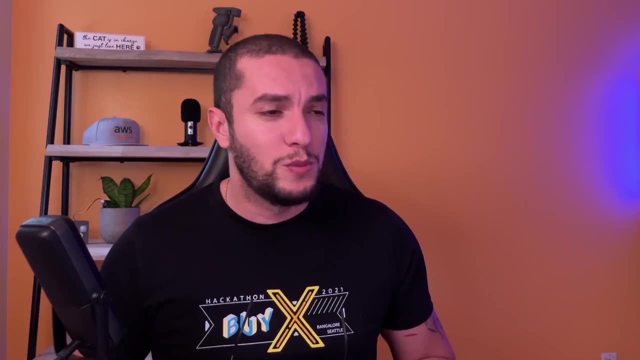 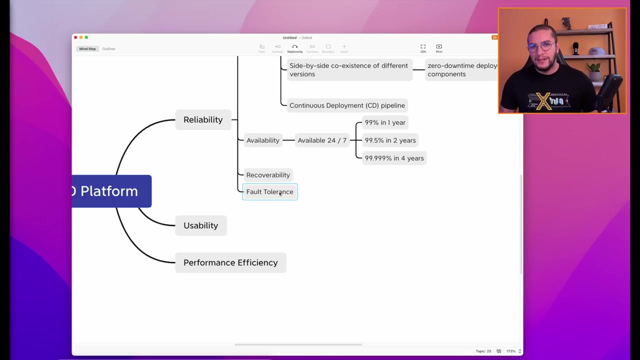 you go and sit with these people, stakeholders, and you negotiate these things with them And you make sure to find that sweet spot where everyone is comfortable and everyone agree to move forward. Moving next, let's touch on the fault tolerance aspect of the platform. Fault tolerance basically means that our 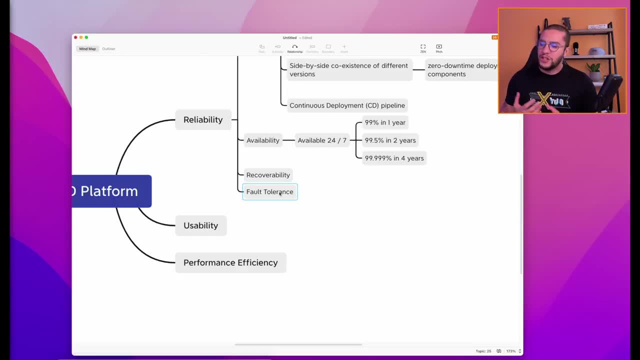 system has no service interruption. So how can we achieve this fault tolerance? In my opinion, one of the best ways is to have resilience built into the system. So I want you to go talk to the right stakeholders and ask them what are the core functionality that must always be on? Of course, we want everything to. 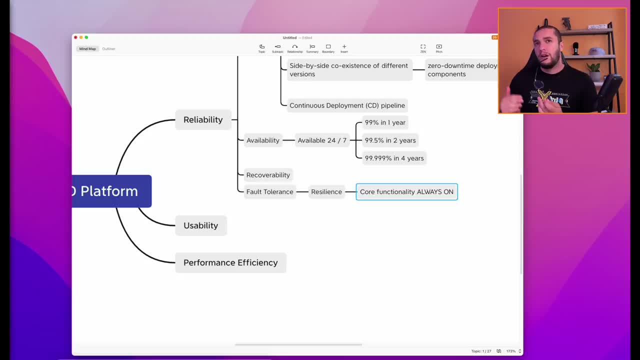 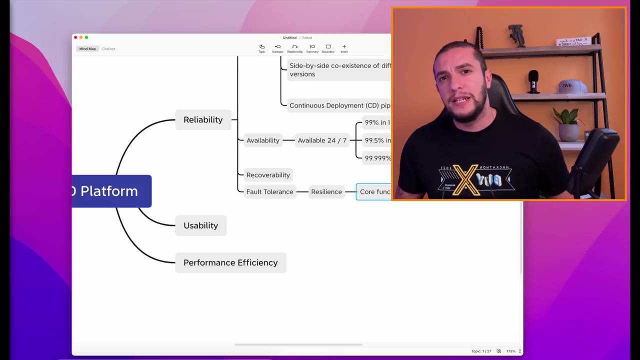 always be on, But usually fault tolerance and cost. usually the higher fault tolerance we want to achieve, the more expensive the system gets. So again, you want to get to that sweet spot. For example, talking about the VOD platform, I would say the ability of uploading videos, that's a must, That's a core functionality. But 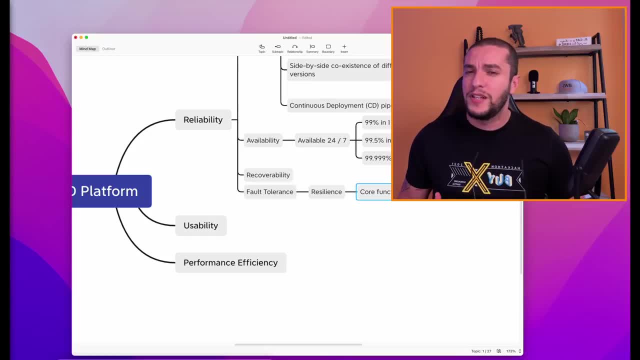 sending notifications. maybe we can afford this feature to be down a couple of minutes a month, and, of course, we need to design it in a way that, when the system comes back on, or when this service comes back on, nothing was lost. You see how, now we touched on the negotiation aspect that comes out of 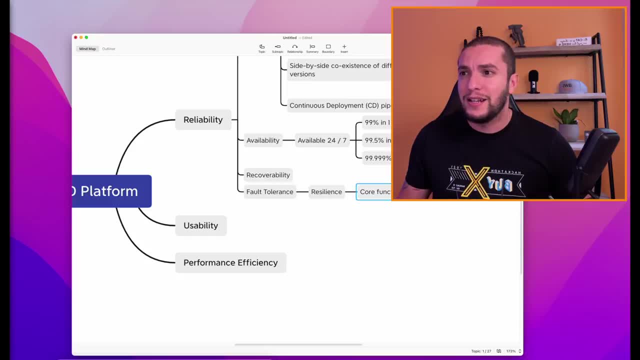 this document, but also it helps tremendously when you start designing and we start choosing the services and we start choosing the architecture that you're going to be using to design this platform. So let's keep going Now. we want the core functionality to always be on. We want also for this: 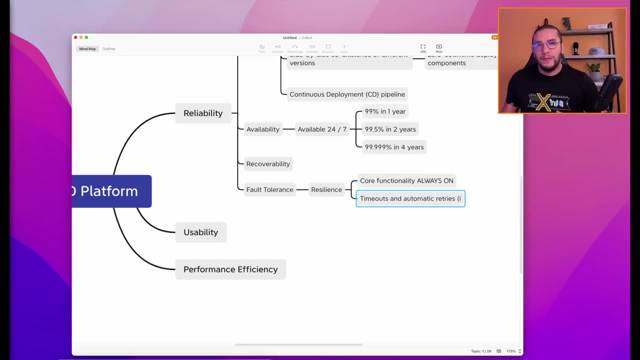 specific example, to have timeouts and automatic retries. because- and something that I touched on on this specific video as well- When you build a distributed system and distributed micro services system, where one component is making calls to other components, you include or you insert the network aspect there. so in case of 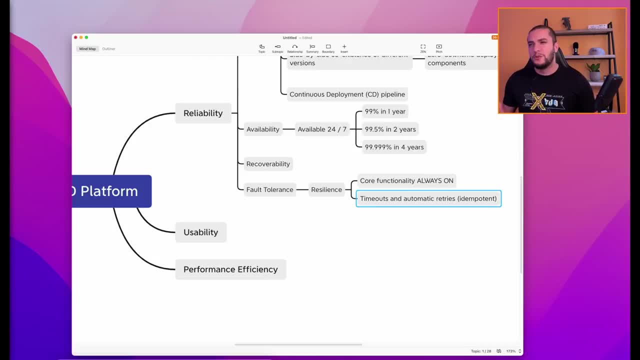 failure, you want to be able to retry that call. you want to be able to wait a little bit and make a different call again, but you don't want to keep making calls just until you exhaust all the resources. so this is something that you need to think about when you're building a resilience. 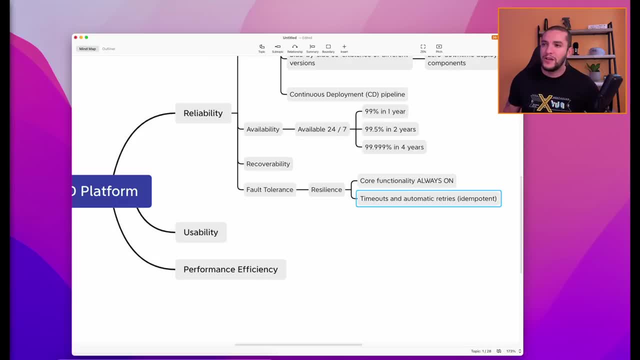 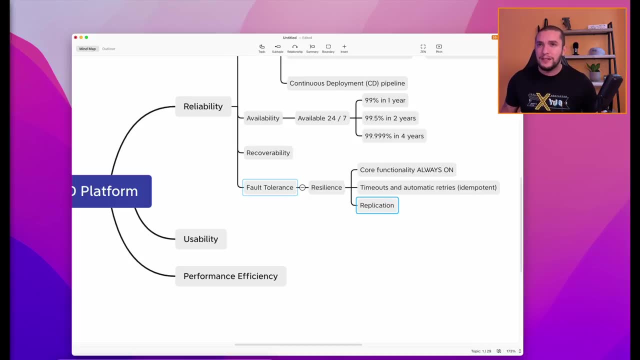 into your application. it's something i touched on in the serverless pattern series, so make sure to check that as well. replication is a big, big aspect of resilience in my system. of course i want to replicate my services and get closer to clients, to customers- but it comes at a cost as well. so 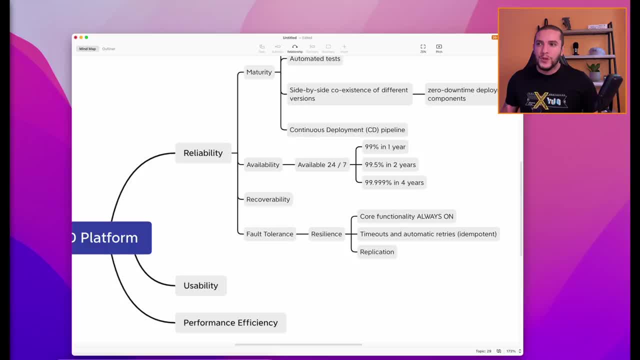 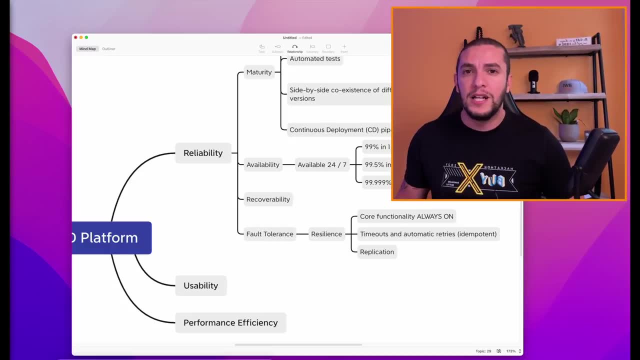 this is something i want to be mindful in when i'm talking with my stakeholders and include them in this design process and these decision makings, and i also want to be mindful of it when i'm choosing the right services and when i'm doing my recommendation. should we, for example, let's 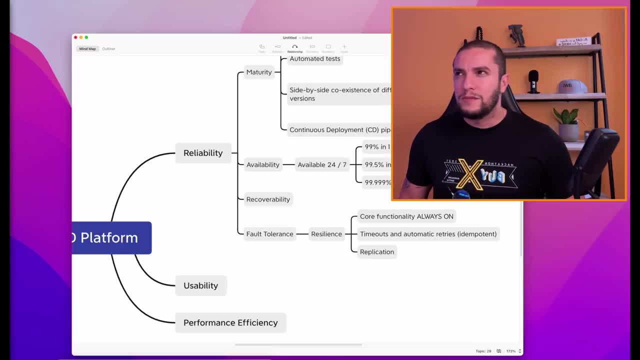 talk about replication for databases. should i go with a global database or should i go with just one database with multiple raise replicas? what kind of read replicas do i need? what kind of read replicas do i need? do i need to have a replication on the master notes as well, or only on the you? 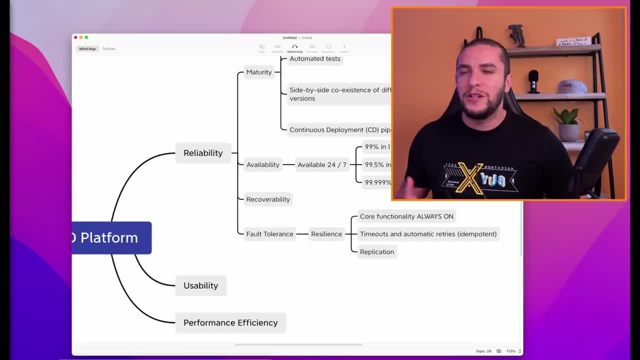 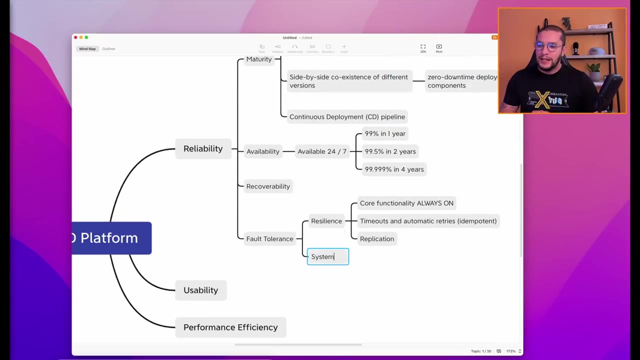 know reads. so in talking to, for example, business people, you're going to be asking them: where are the users located, what is the latency that we can afford, and you translate their answers into decisions that are going to help you making your own designs. system overload is something i used to do a lot before- not very much now, because i pretty much 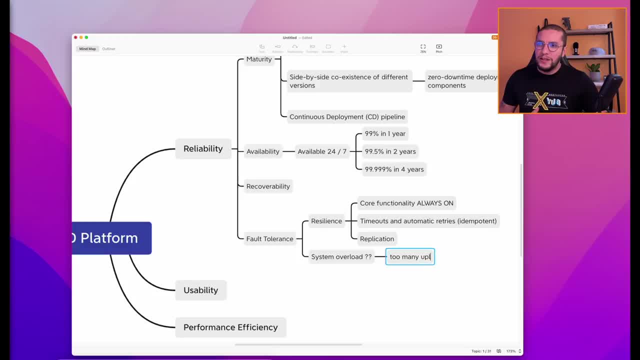 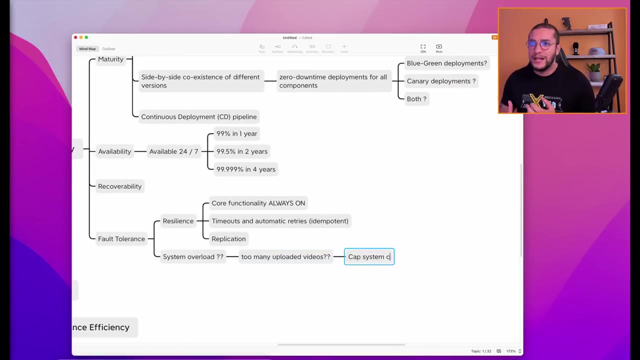 use a lot of莳 serverless services currently, but I used to want to overload my system until I break it. and once I break it, I know exactly the threshold where it breaks at and it allows me to add alarms beforehand, like at 70%- 80% of that threshold, I start sending alarms, I start waking up people. at 2 am not me. 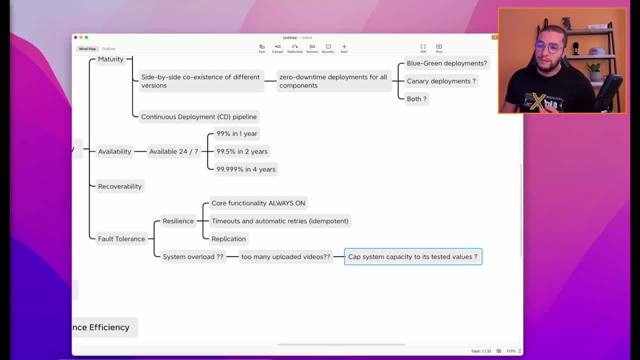 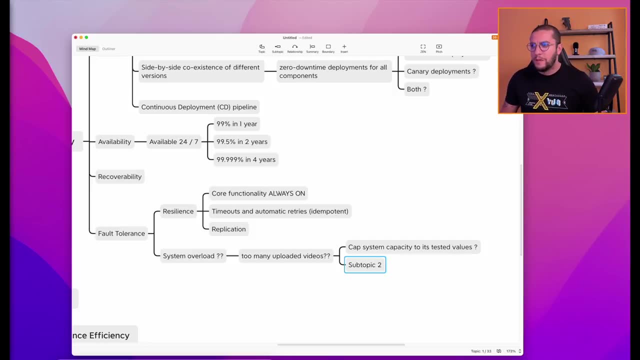 manually, but pipelines that I design into the system, like cloud watch, alarms using the cloud watch metrics and other steps that are out there. so what happens when there are too many videos being uploaded and we start reaching that cap, right, that threshold? I will design two separate processing queues: one with a higher power for premium users, users who pay a monthly fee, or 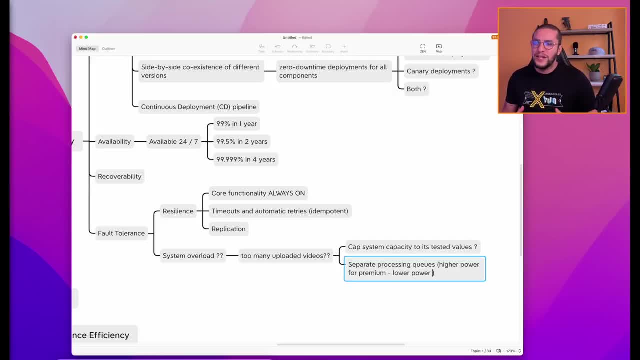 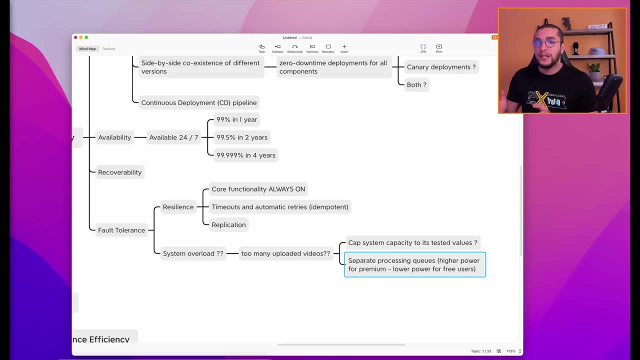 whatever. and then another queue that is a little bit slower for users who are not paying right, and it's just one way of solving this: decoupling the processing power and giving more power to the system. and it's just one way of solving this, decoupling the processing power. 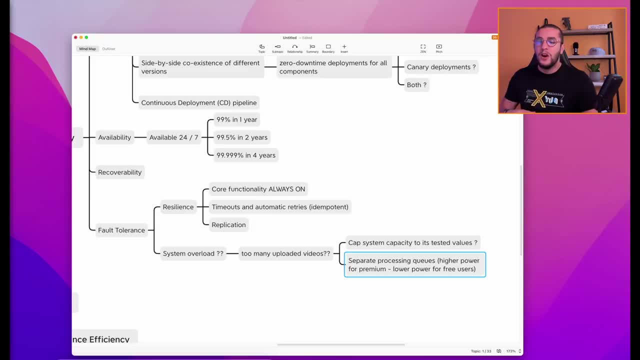 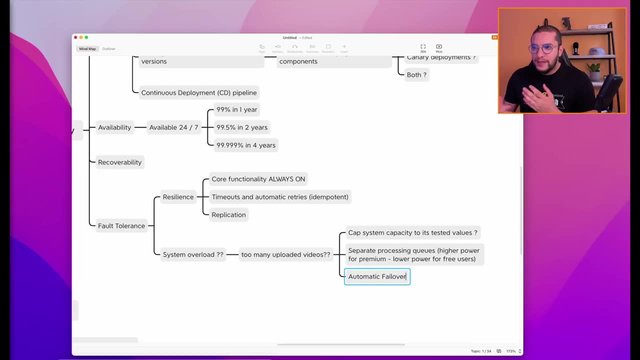 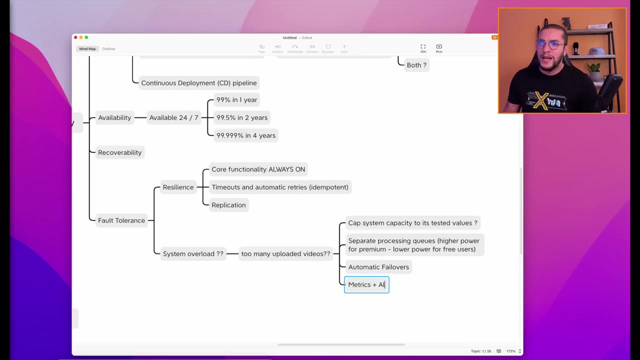 power to premium users or closer users, or farther users or loyal users. you get to choose. I also want to build automatic failovers into my system. it's at this point that I start thinking about the disaster recovery strategies that I want to include into the system and I go talk with the ops team. 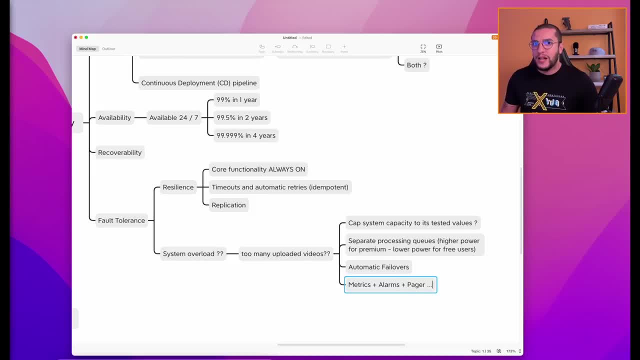 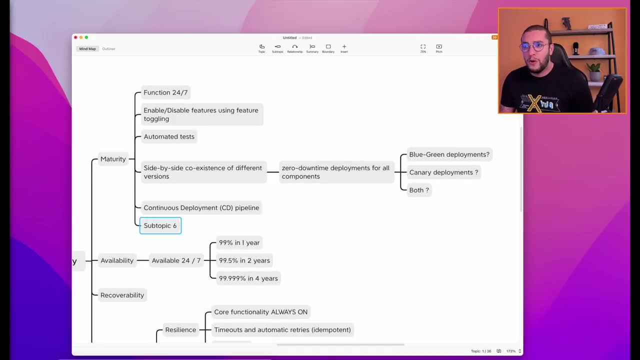 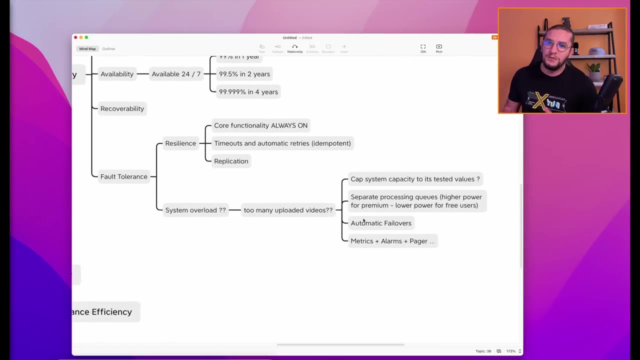 and start asking them about what are their SLEs regarding disaster recovery. I go talk to sales people and I ask them what happened if the website goes down for more than 10 minutes. are we going to business? is someone going to be fired, you know, or is it? no, it's fine 10 minutes, we're going to be okay. and 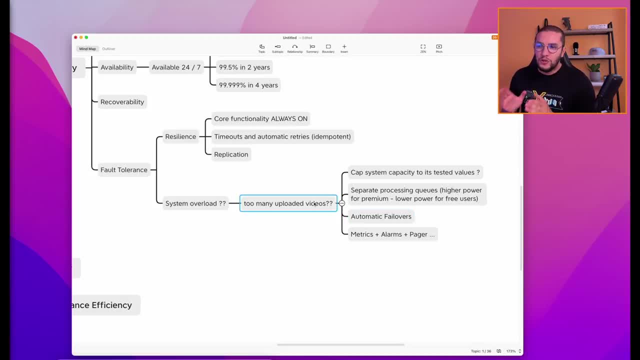 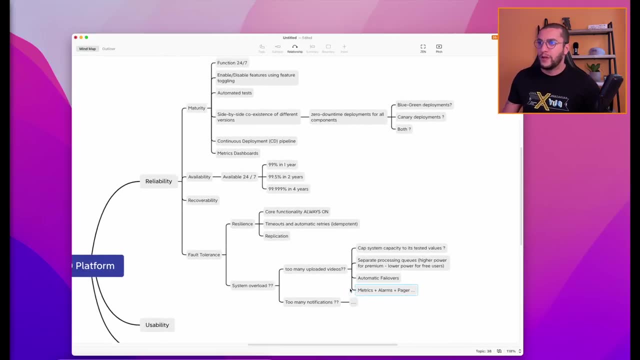 we'll just recoup whenever we come back up, and you know it's super helpful to have these questions and have these answers before you start designing the system. all right, here we go. so we already know a little bit more about the solution that we want to design before even starting to design it, and 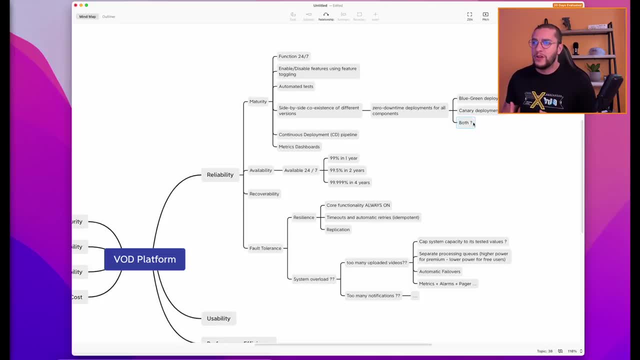 this is one of the other big advantages of building non-functional requirements, and having them listed this way is including everyone in this decision process, and it's really important to know your system. this is a very important process, and so, before you even start choosing your first service, you know exactly how the system is supposed to function and all these small edge cases about it. 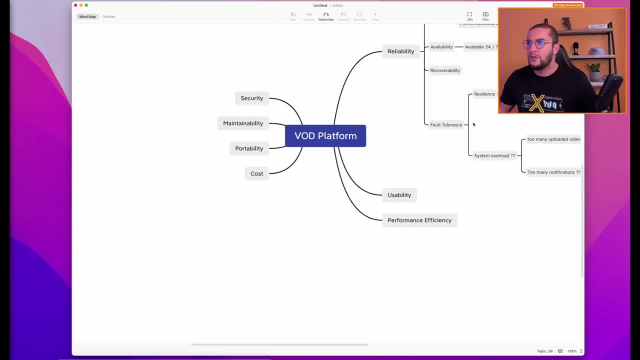 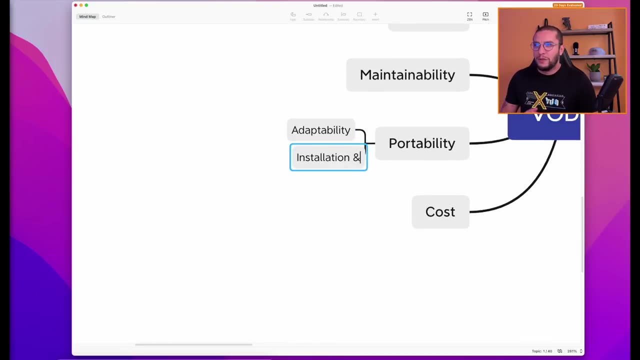 so let's let's go somewhere else. let's look at a different requirement. okay, let's go with portability, so how my system will adapt and how my system will be installed on will be deployed right. and adaptability is about making your platform scriptable and easily deployable and reproducible. 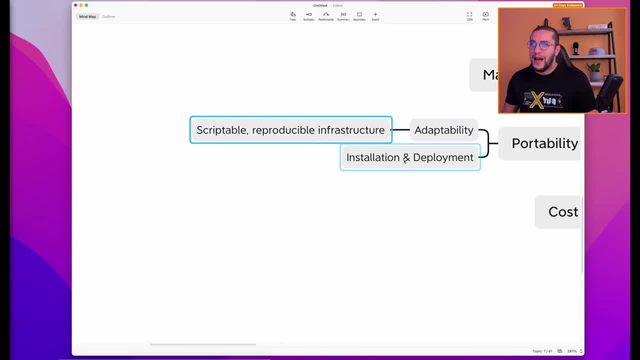 Reproducible in different environments and, of course, how we make this today with today, tools is using Infrastructure as code, and at this point you want to talk with your developers and with your ops teams and ask them: What's framework are they interested in? What's framework do they prefer? right? 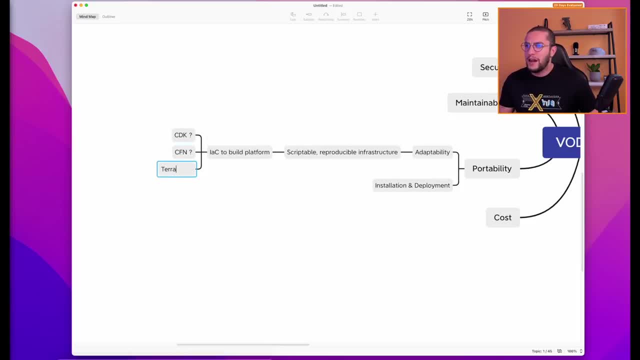 We can do this with CDK, CloudFormation, Terraform and a lot of other ones, But everyone, every one of these frameworks, has its own Limitations, so you just want to be mindful of these limitations before you start Designing your system to be scriptable and to be reproducible. and another aspect of the adaptability is the auto scaling and elasticity. 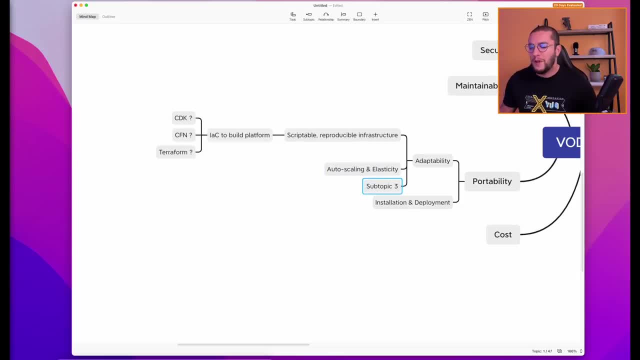 Of course, if you go with something like serverless, you don't have to think about this much. But there are always caps. the cloud is not infinite, even though it seems like it, so you need to have these points Raised before you start designing your system. now moving into the installation and to the deployment aspects of the application. 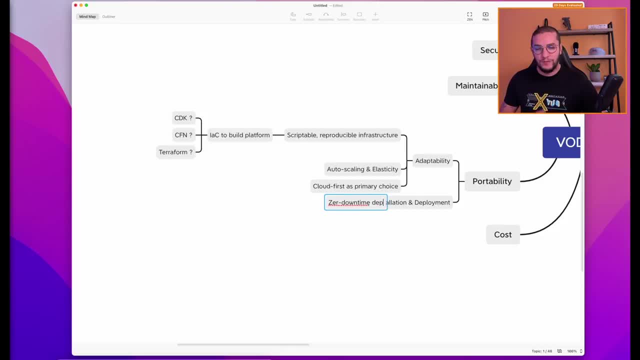 Of course we want to introduce a zero downtime deployments 24: 7. We wanted to Automated. so this is gonna help me when I design my solution and design the components into solution to get updates 24-7 in a zero downtime fashion. So remember, beforehand we talked about the ability for multiple components version to exist at the same time. 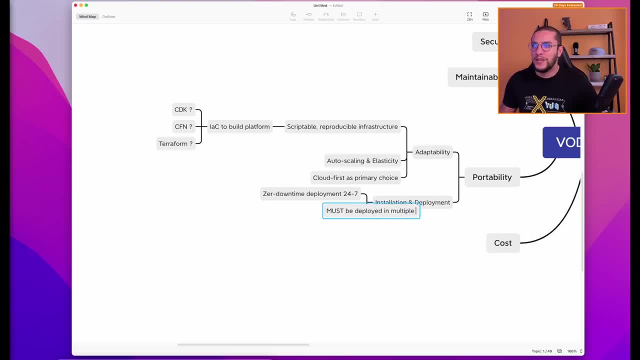 So this will help as well. We also want the system to be deployed in multiple AZ, so we want to take advantage of the multiple availability zones and the different regions that AWS and other cloud providers offer as much as we can. These are super helpful features if used in the right way. because, yes, 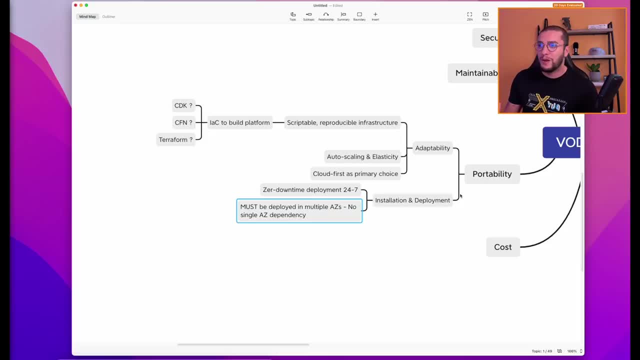 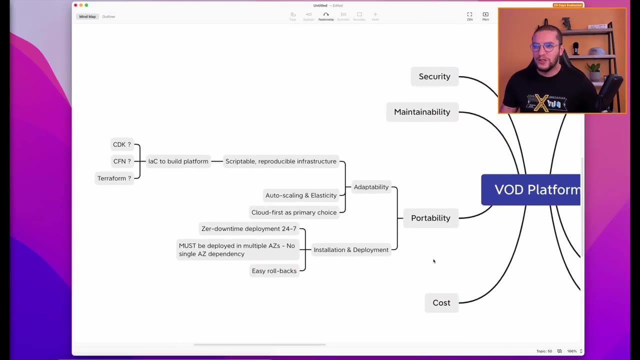 the more your replicates, the more money is gonna cost what's worth it to your company, and usually companies gets a lot more from Being multi AZ and multi region than you know what what it cost them to be there. I want to also my platform to have rollbacks, and you want these rollbacks to be super easy. 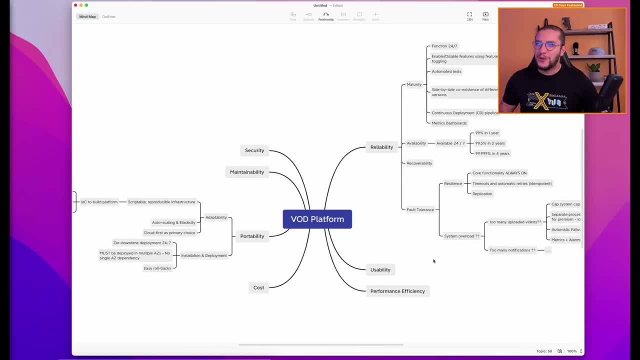 All right, so we touched on a few already. I can't go through the hundreds plus Environments that usually gets added here, but you know what? Let's add a couple. So let's touch on the cost and add just a couple of notes here. We want to know the cost per environment and 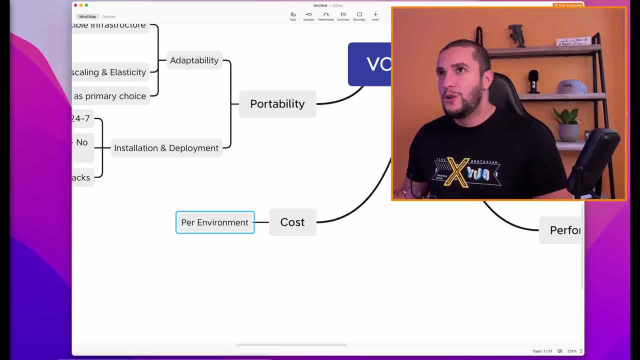 Why? because this will lead you to usually the marketing people, because they know they would give you numbers that you need. How many users are we expecting after we launch this fall? How many users are we expecting in the next two years? right, And although you're not looking for the exact number, just looking for a ballpark. 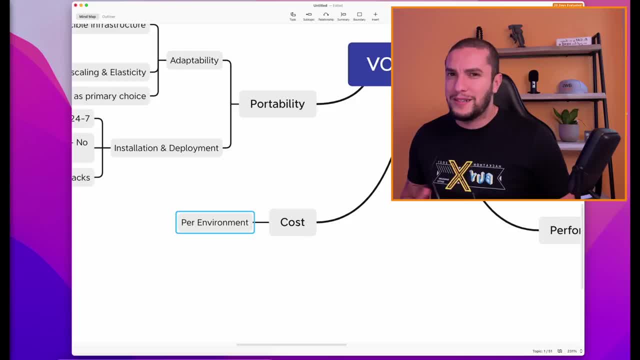 You want to design your system to be scalable, So you need these numbers right. Or maybe you talk with salespeople and see how many purchases do we get per second, per month, per year, per six month, per minutes, per hour, And that's gonna help you calculate the cost. How many databases do I need? 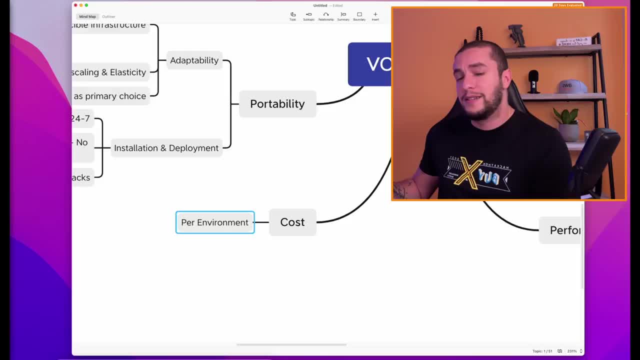 Maybe it's better to go for a NoSQL database because of this, this, this and disadvantages. Or maybe I just need three replicas if I'm using a relational. Oh, maybe I need an OL app for this and it's gonna help me cost rather than having six OLTP. 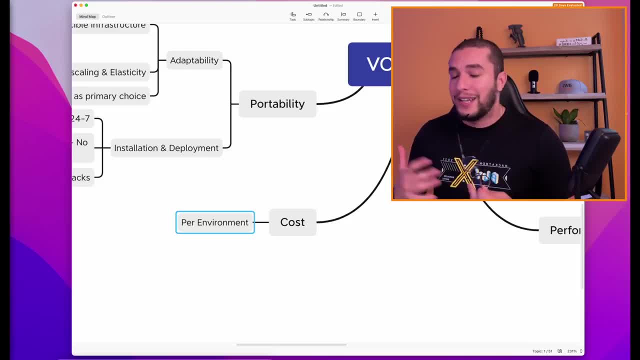 databases- this really having all these questions again, i keep repeating it- but this exercise is really a goldmine and it helps you tremendously before you start choosing, because sometimes two years later or three years later and someone asks you: why did you choose this database? why did you? 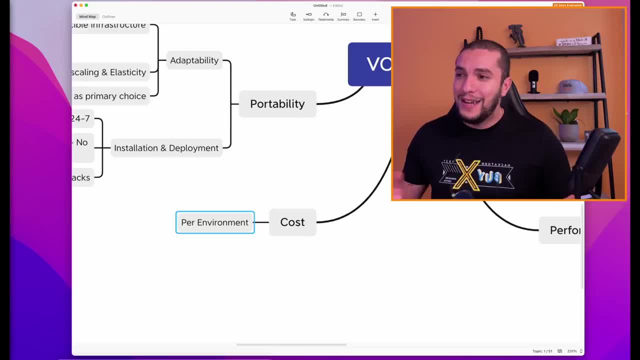 choose that other one, you'll be able to come back and say, hey, when we built this thing, here are the reasons, here are the requirements, the conditions that we have, the realities of our business at that specific time, and this is why we did it that way. if you only have the final design, it would be hard. 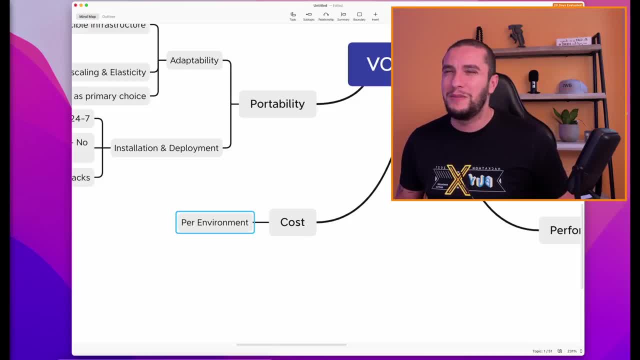 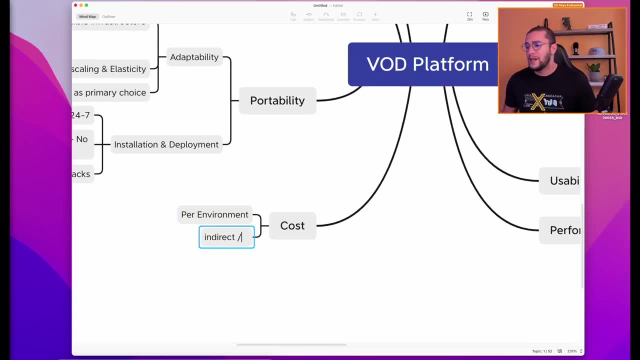 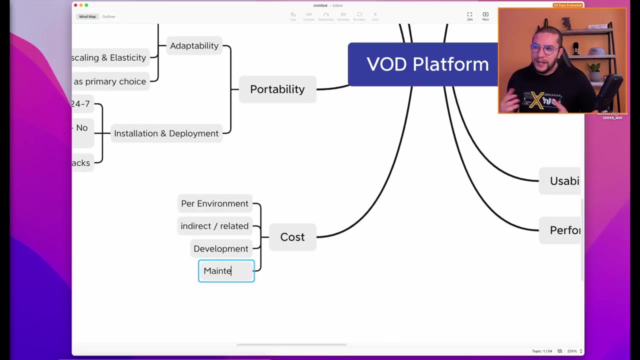 in five years to say, oh, we only choose my sequel because i don't know. you know you don't want to be in that position. the development also and the maintenance also has a cost, right in time and in money. you want to choose, probably services and an architecture that your technical people in house. 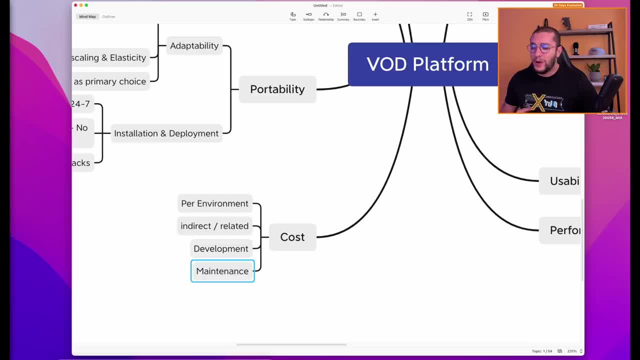 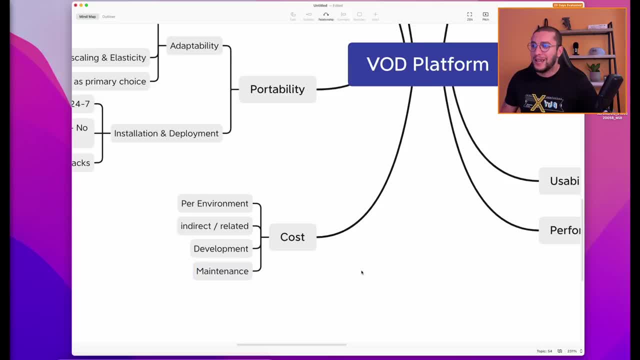 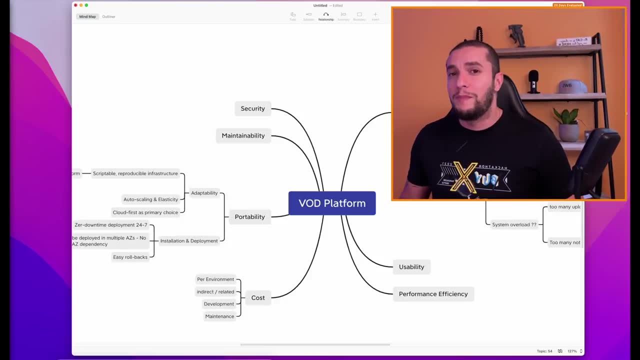 latest shiny framework no one know how to maintain because that's going to cost you a lot maintaining it, even if sometimes it's the right solution. it's really rare when we apply the best engineering solution because we're not living in a bubble. my solution is not built for engineers by. 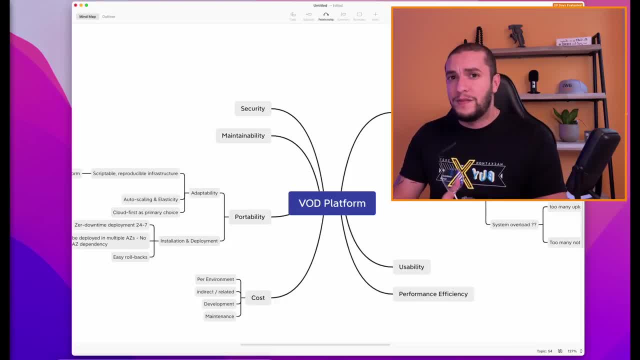 engineers. it's operated by people, built by different type of people, consumed by different type of people, being paid for by different type of people. so you need to include all these decisions into building and you need to include all these decisions into building and you need to include 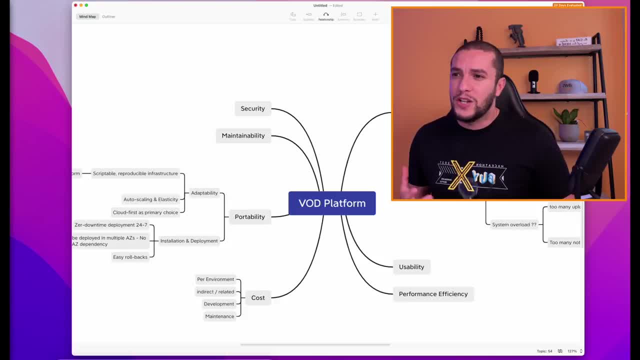 it's fine to make compromise right and, as i mentioned before, we try to build these things in iterations- we're engineers, after all- but you just need to incorporate all these things into your decision making. and the last component i want to touch on in this video is the maintainability. 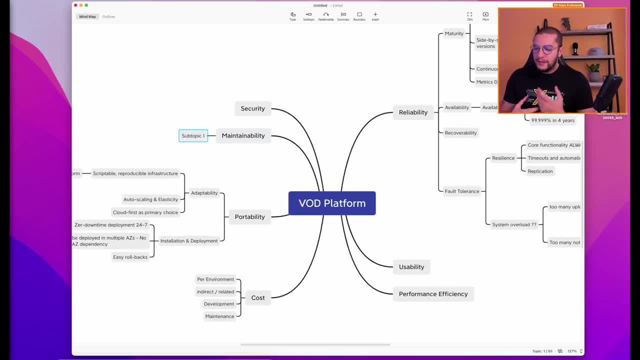 aspect in the maintainability realm, we try to define how easy it would be to make repairs on the system, how easy it would be to introduce something new to the system. right, and as i mentioned in the previous video, we talked about how easy it would be to make repairs on the system. 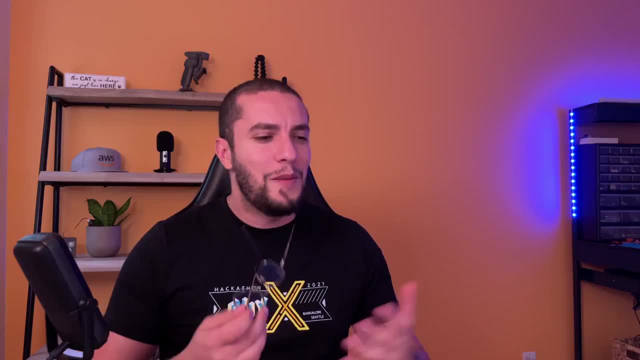 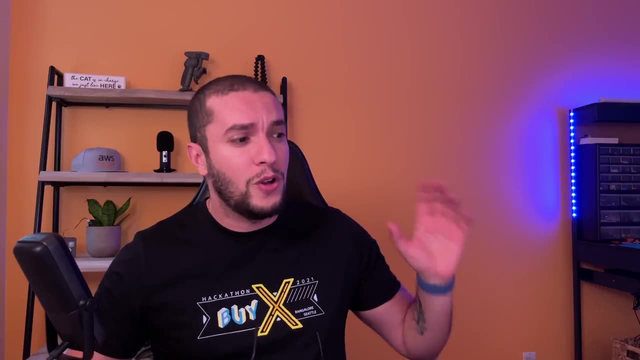 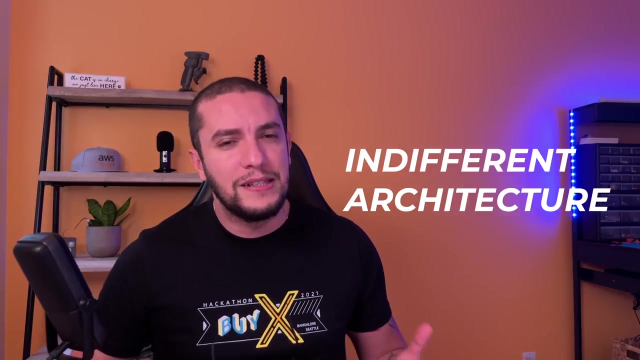 in various videos, probably before that, building a system that works. that's easy, right. you can just download the framework, follow the framework documentation. they say: put all the controllers under the controller folder, put all the models under the model folder and it would work. right, that's what we call indifferent architecture. it works, it's great. it helps you to go from. 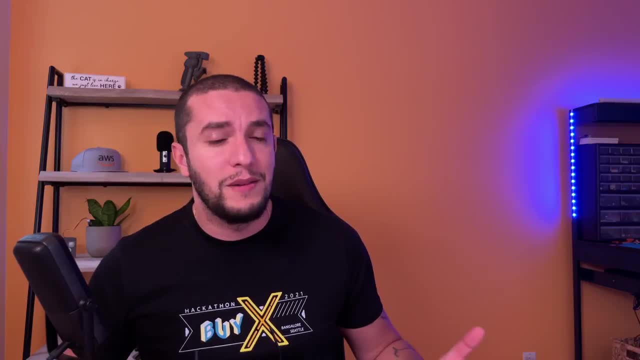 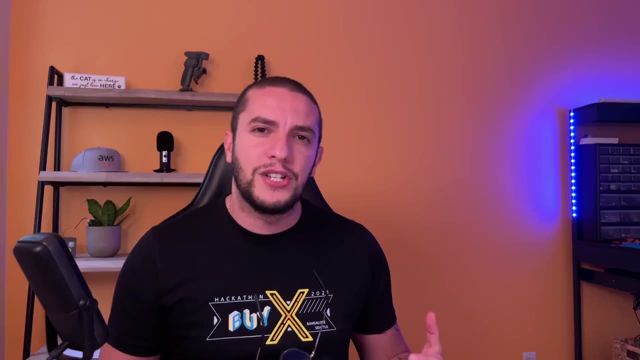 you know, point a to point b: go to market quickly. i never thought anything bad about monolithic frameworks. i'm not thinking they're evil or whatever. they actually serve their use case. their problem is actually their maintainability ratio, which is super low because it's deployed as 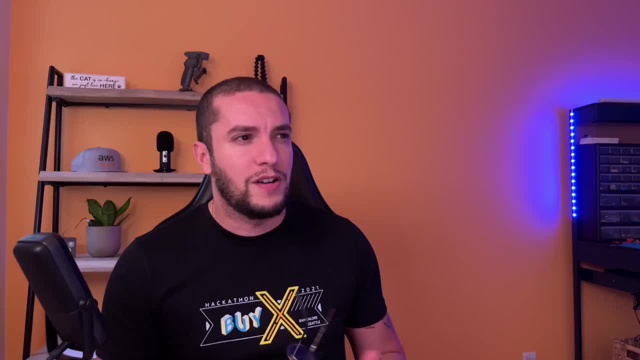 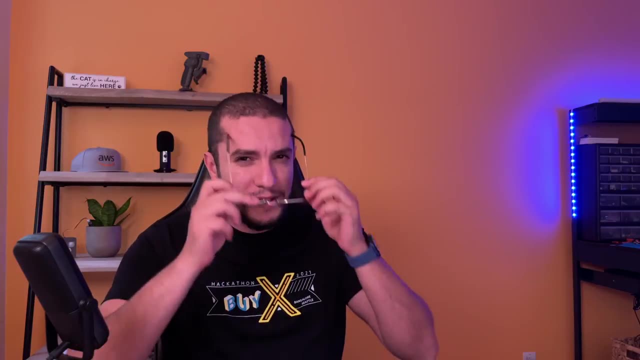 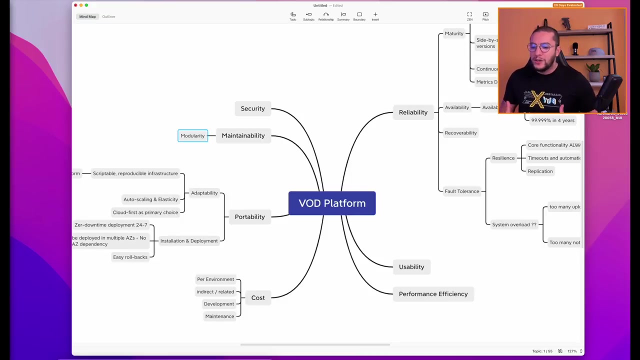 one big piece and it's. it's not modular enough, right, especially after a few years. so building a system that can be maintainable for 5, 10, 15 years, that's the the hardest thing. one solution that we tend to use to increase the maintainability ratio is to use modularity. i want to design a 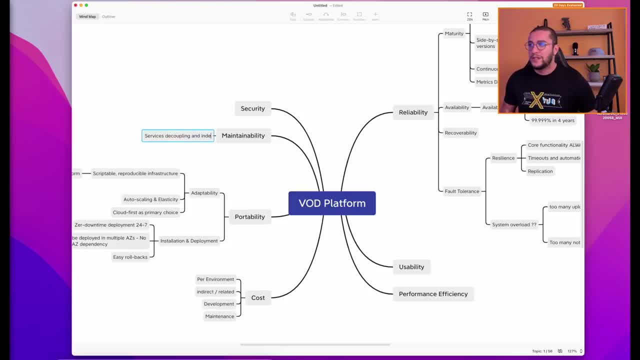 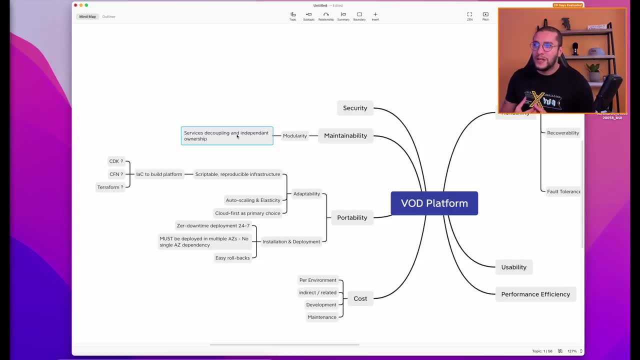 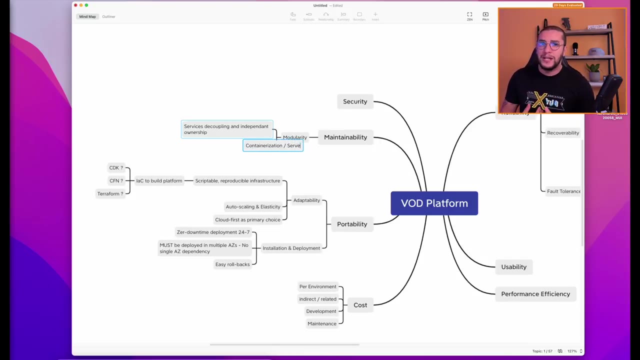 system where services are decoupled and where services can be owned by different teams. so you see how now this is giving me actually more data and more insight into how i need to design my system. probably i want to use containerization if i know that my company has a lot of experience. 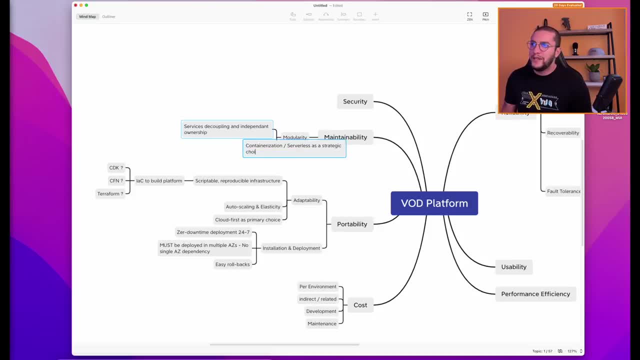 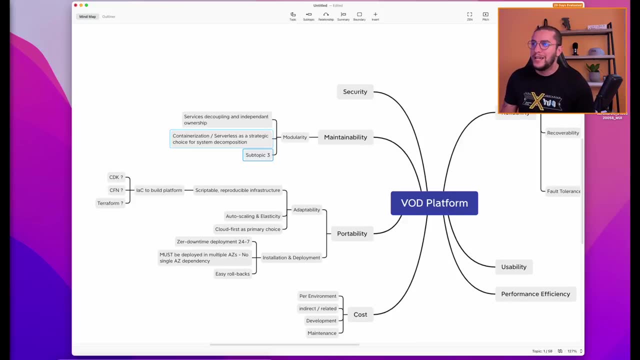 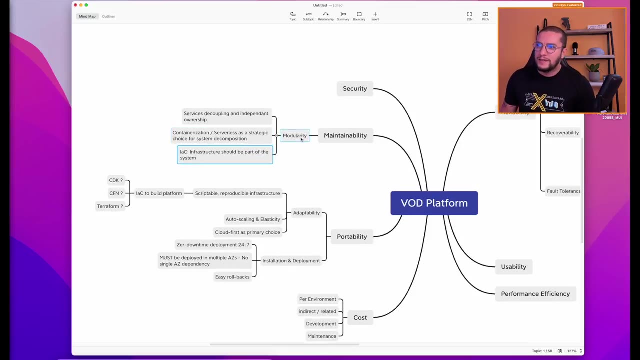 in containerization. am i going to use serverless again? you, this is where you make your strategic choice for system decompositions, and you do that by talking to the various people again and including them in this decision making. um, infrastructure, as gold should always be part of the system. right, and there are other stuff that you could add. 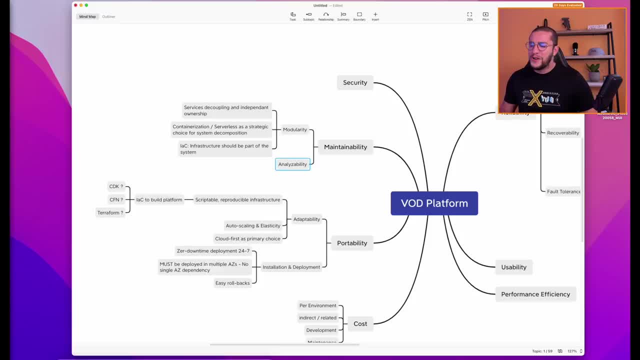 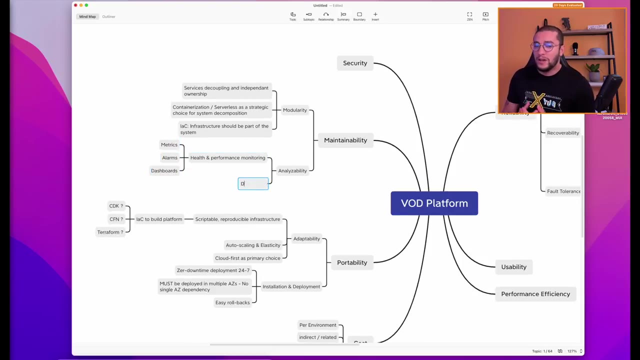 as well. there for the analyzability- i never know how to pronounce this- you basically need to design an architecture where it's easier to have a performance monitoring and health dashboards and stuff like that for various systems and services, right, but also as a whole login needs. 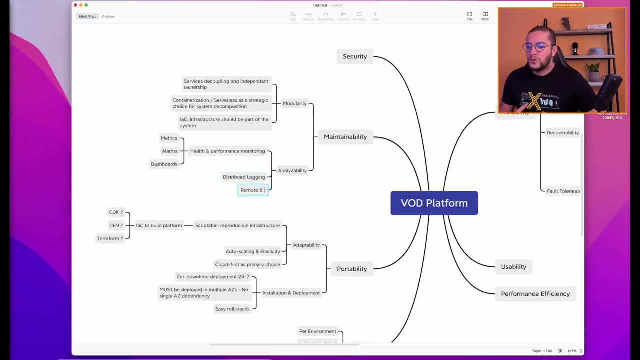 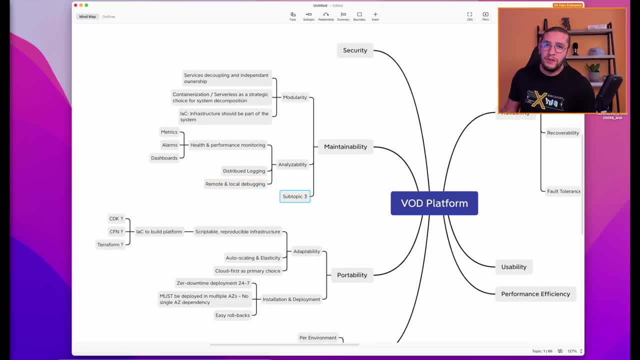 to be distributed as well. sometimes you want to offer remote debugging to your development teams. sometimes it's not necessary because it's just gonna cost a lot and it's not really worth it for them to have a system. and in this case, what else we can add into the maintainability here? well, 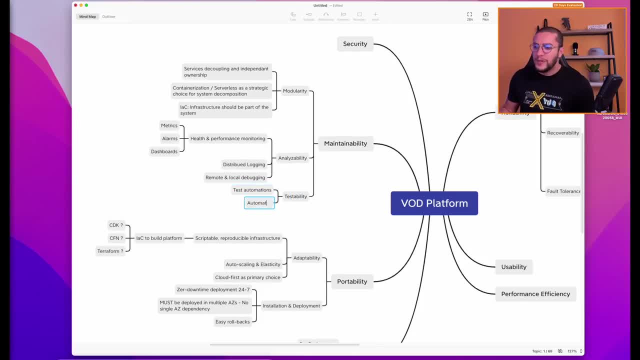 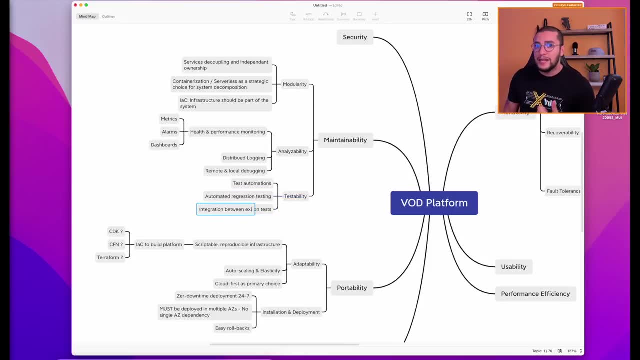 testability right, how? what is the kind of coverage that we have into our code? can we test the components separately? if not, i need to design actually a system where components can be tested separately and they can also be tested when they get integrated between themselves. i need to also 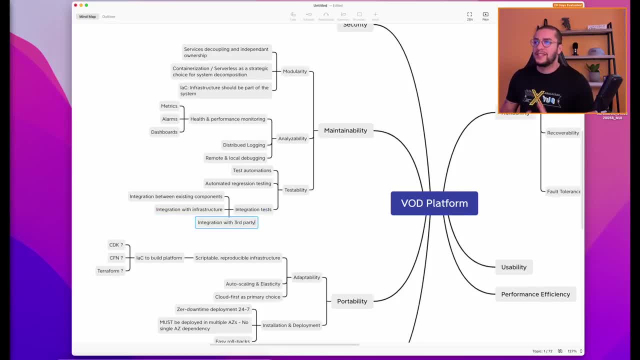 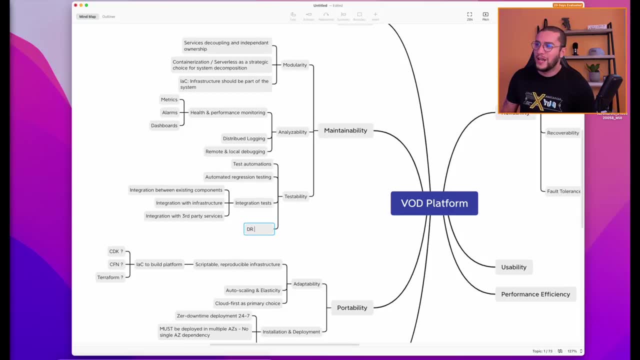 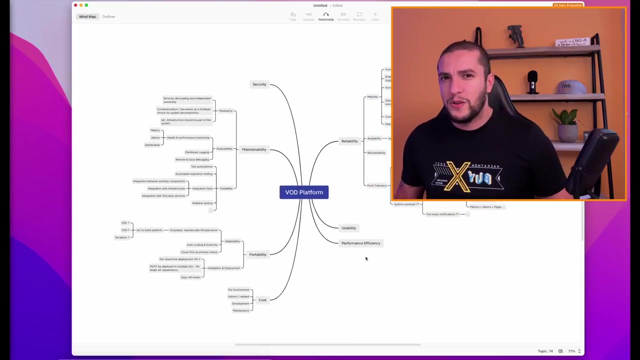 design a system where i can test deployments, where i can test rollbacks, where i can simulate um disasters right and test rollbacks, and ews has a lot of tools, engineering and stuff like that that would help you definitely build solutions like this. and that would be all for this exercise. my goal was that to share the workflow that i go through before i even